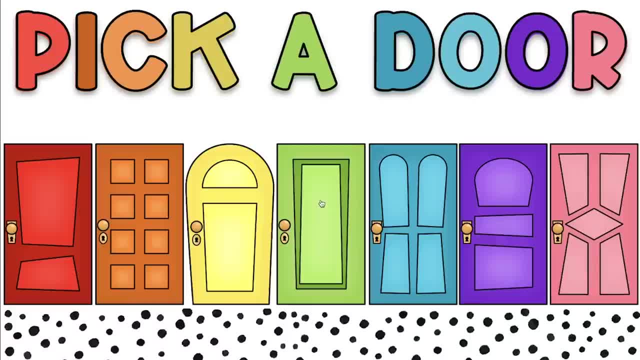 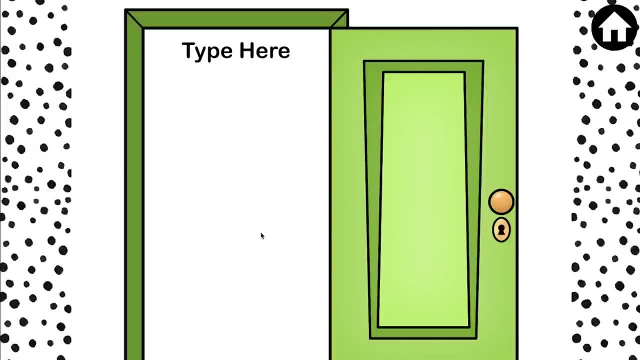 they'll have a question that they need to answer and you'll see a check mark pop up like this: So let's say, a student picks the green door and here you would have the question ready or a visual or something that you want them to answer, and then click the home button to go back and you'll see. 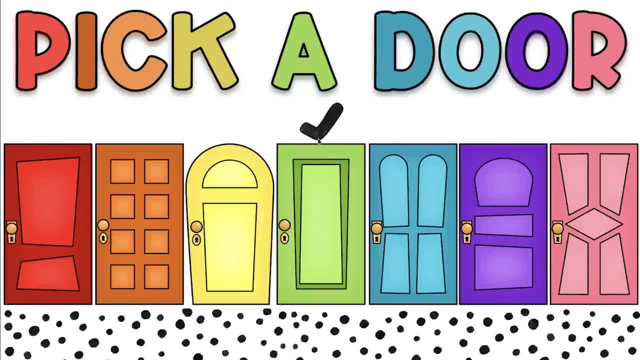 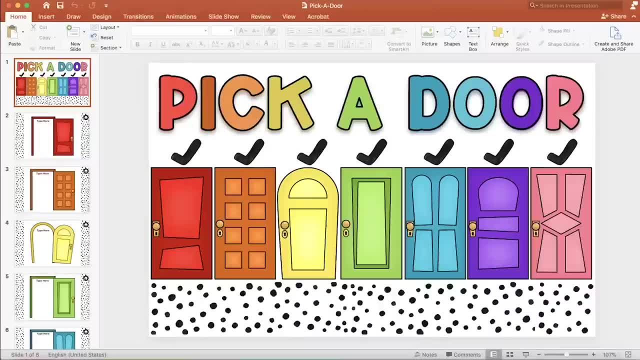 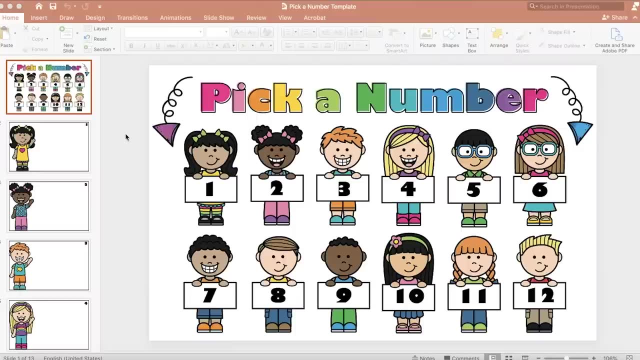 the check mark appears so that the other students don't pick the same door, And that process will repeat every time a child chooses a door. I will have this interactive slide template linked below this video. Now I'm going to show you, step-by-step, how to create a game on your own, just like this one. 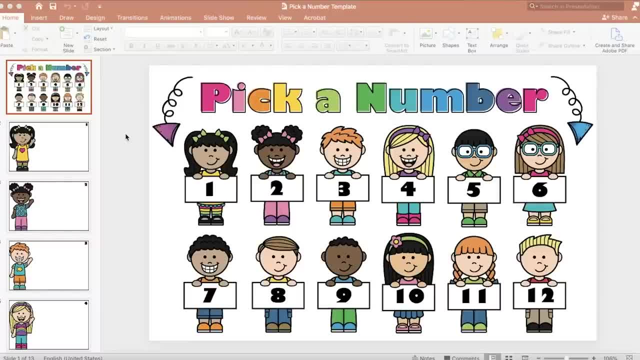 This is so you can continue to create more games and maybe in the future you'll want to have different themes, or perhaps you want to choose clip art that you know your kids will enjoy. Everything I used for this game called Pick a Number is free: The font, the clip art of the kids. 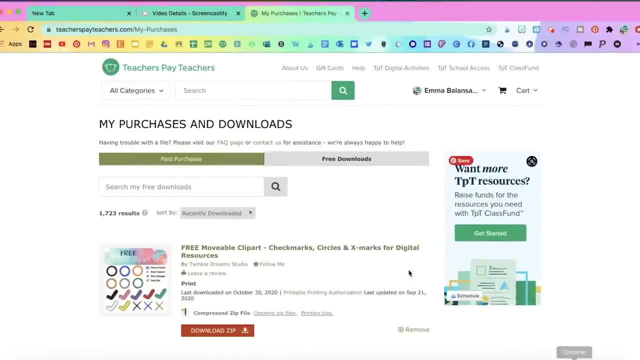 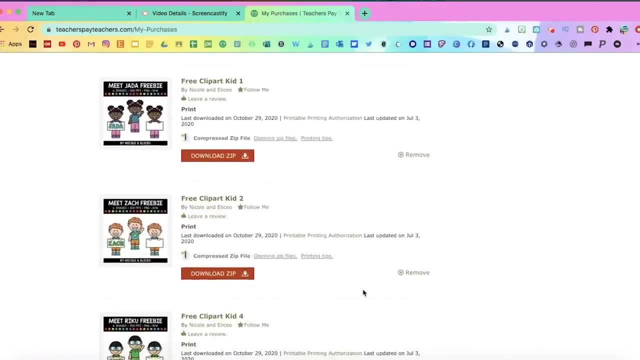 it's all free. As you see here, I downloaded the clip art from Teachers by Teachers, and I'll go ahead and add links in the description below. If you're interested in learning more about this game, you'll find that I have the link to something in the bottom of the video in case you want to follow along. 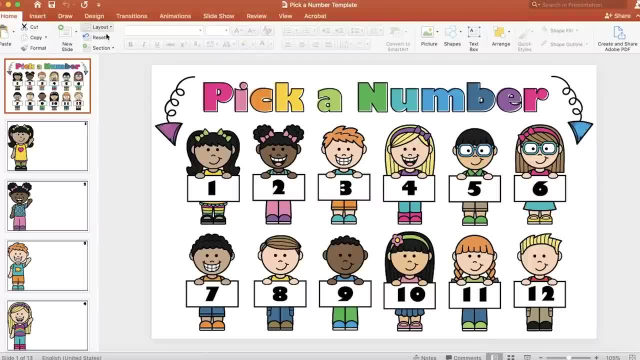 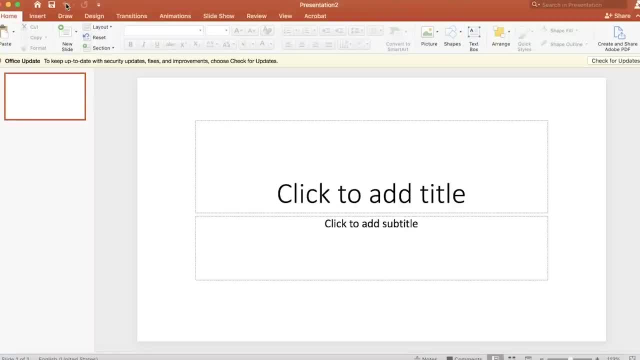 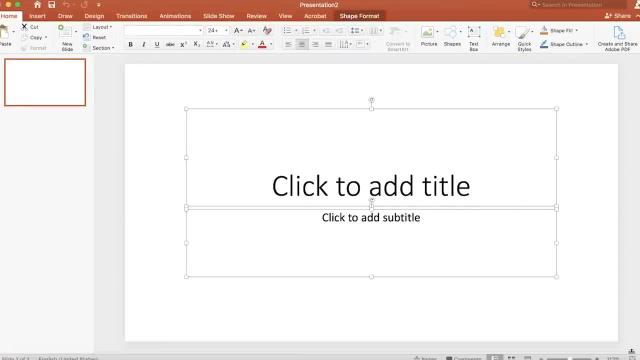 Okay, the first thing you're going to do is start a new presentation. I have Powerpoint open. Then I'm going to go to File New Presentation and I'm going to erase these boxes by highlighting everything and hitting Delete. I'm going to change the size of the frame here. I'm going to go. to Page Setup. I made this a 7Rx Bethlehem-based video, and here it is, within the page size that I have także made a replication of this video. this is in practice, way more process than in my previous video. I've bitterly)] a Nederland varqa, которое me dat alternat��igrade werden, dan ik yolkanna. 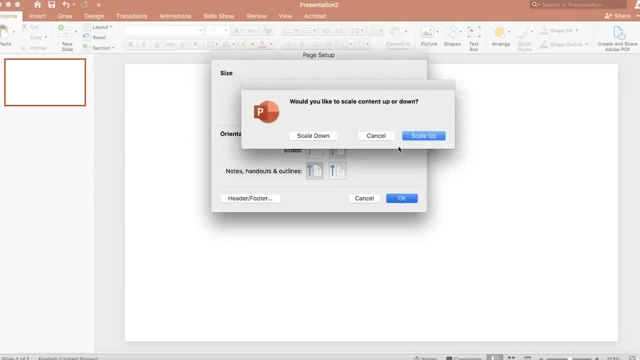 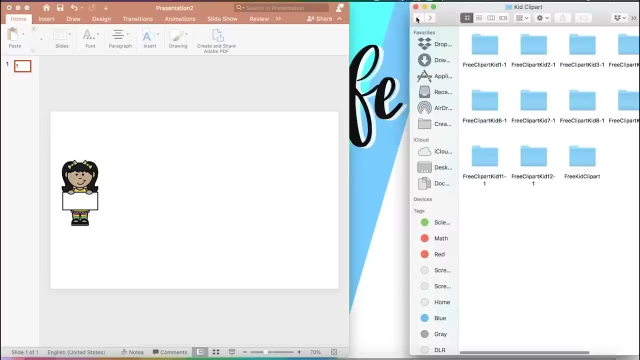 13 by 8.. Okay, so what I'm going to do now is drag all of my clip art to my PowerPoint. I'm going to start by putting the kids in order into two columns, I mean into six columns and two rows. 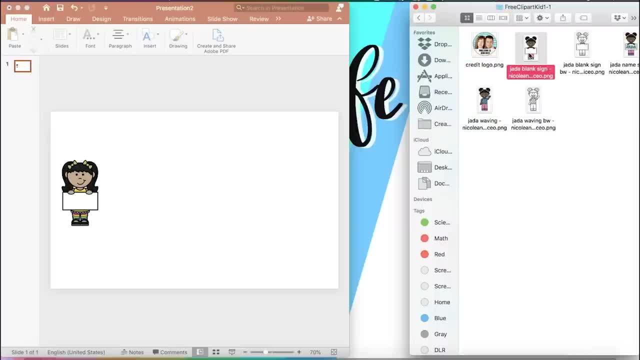 and what you're going to do is open the folder and choose the kid with the sign and drag it, and you're going to pull the corners so that it's the same size as the other kid and you're going to see these lines, these red lines, pop up. That means that they're both the 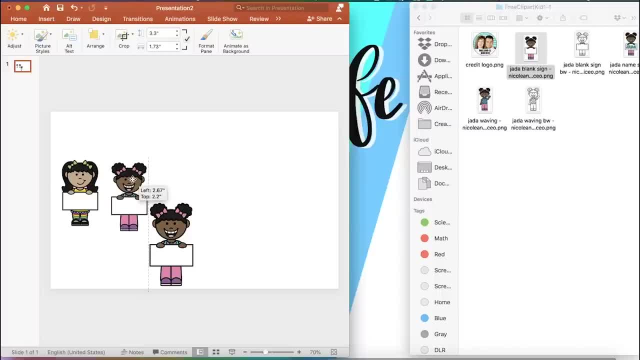 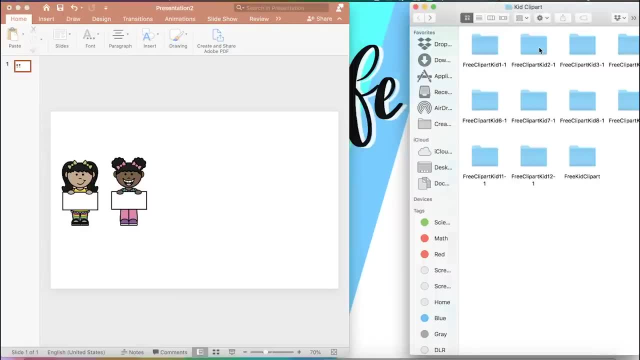 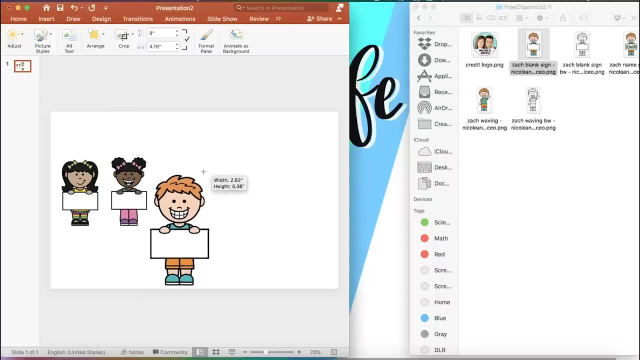 same size and width and that's exactly what I want to do, so that they look similar. and then I'm going to go back, go to another folder and then drag another kid and then you'll see that when I pull the corner down, as soon as it's the same size. 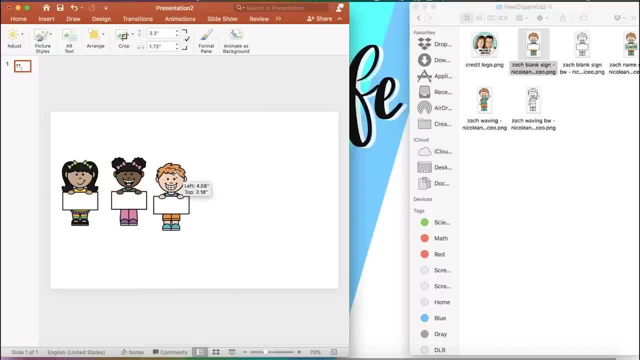 as my other two clip arts. it'll show those red lines- and this is what I like about PowerPoint: that those lines are very helpful when you're designing something and it helps keep everything very organized. and you're going to follow the same procedure for each clip art, for each kid. 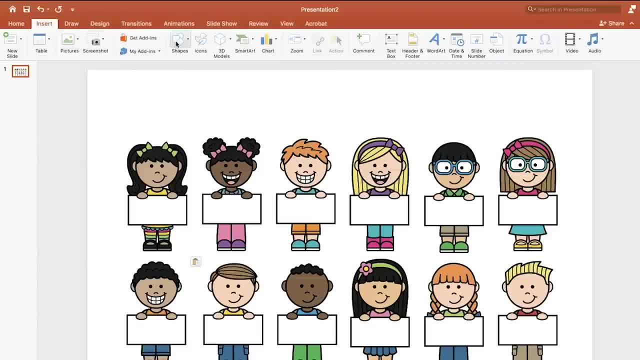 Okay, next, we're going to add the title, You're going to go to insert and you're going to say clip content. You're going to say clip content, You're going to say shapes and click on this text box and I'm going to add the rectangle all. 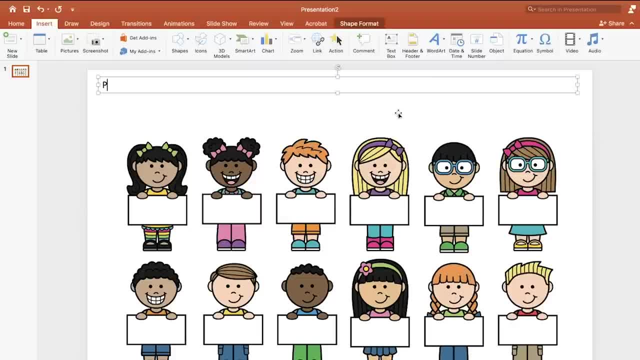 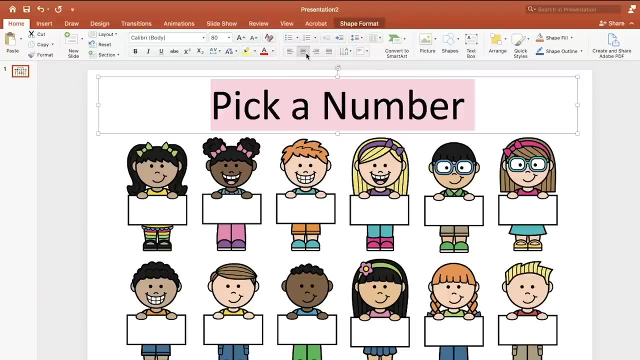 across my PowerPoint and I'm going to type: pick a number. now we're going to change the size to 80, so go to home, go down to 80, and we're going to Center it right there, and I'm going to change the font to a free one called Jill, sans so. 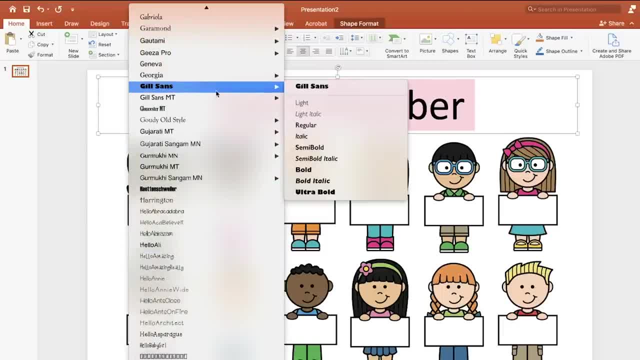 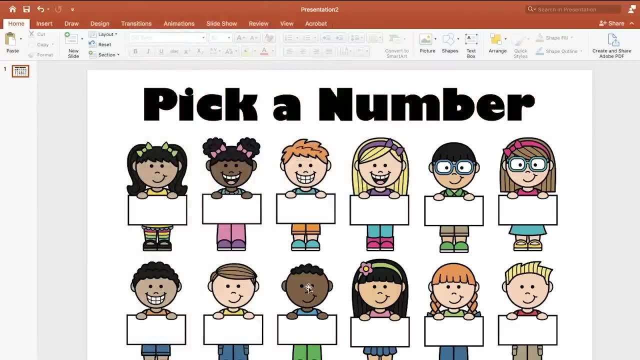 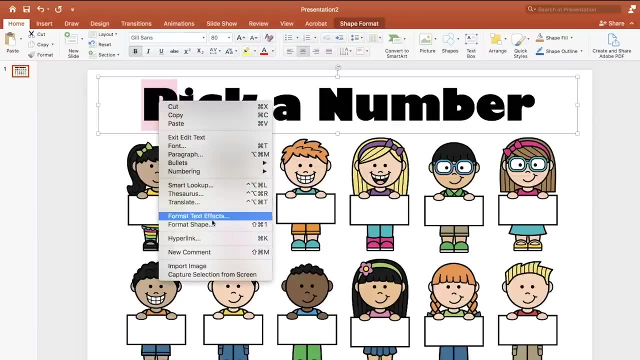 go down to G and I'm going to choose ultra bold. now I'm going ahead. I'm going to go ahead and change the color of each letter. so go ahead and highlight the first letter. go to format text effects. we want to format the text, not the shape. 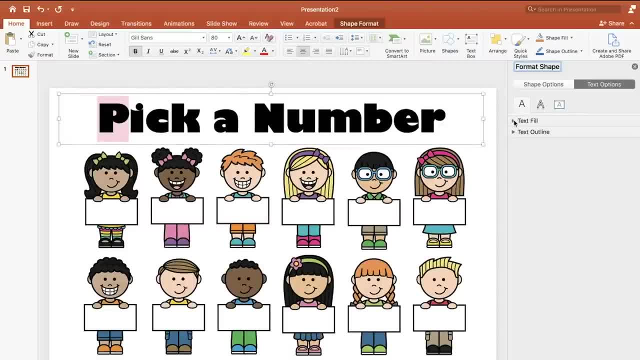 you want to use the font size and then click on this first a, and we're going to change the fill of it. I'm going to create a rainbow, but I'm going to use the colors within these pictures to create that rainbow, so I'm going to go. 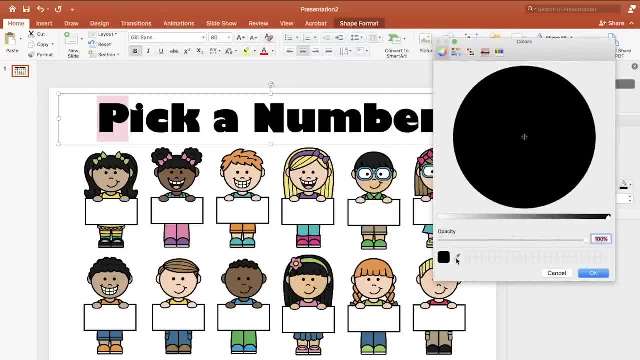 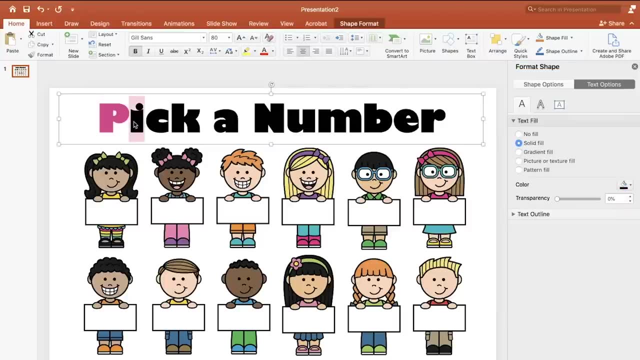 to more colors. slide this over and I'm going to choose this eye droplet here and I'm going to pick a pink. I'm going to choose the pink of this little girl's shoes right here and click on it and you'll see my P turn into that same shade of pink. and then I'm going to do: 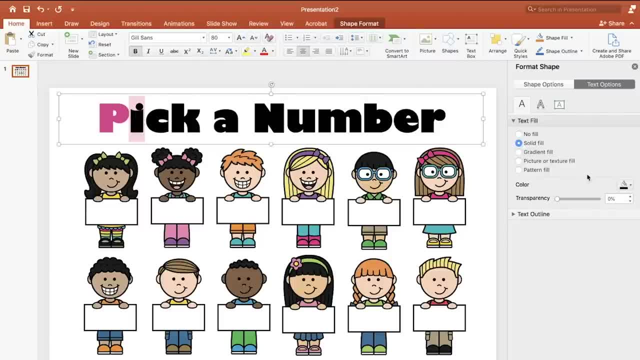 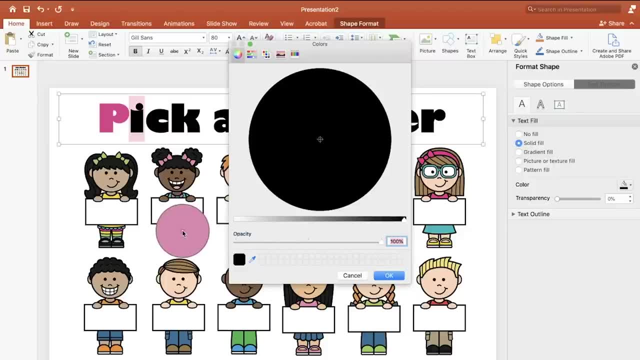 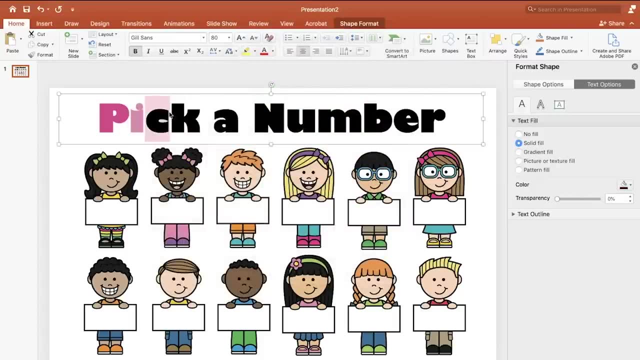 the same thing for each letter and I'm going to follow the colors of the rainbow, um, but using the colors from this picture. now I'm going to use a lighter pink and I'm going to use the pants of this other little girl and then, after pink, I'm going to use- I'm going to choose orange, click on color, go down to. 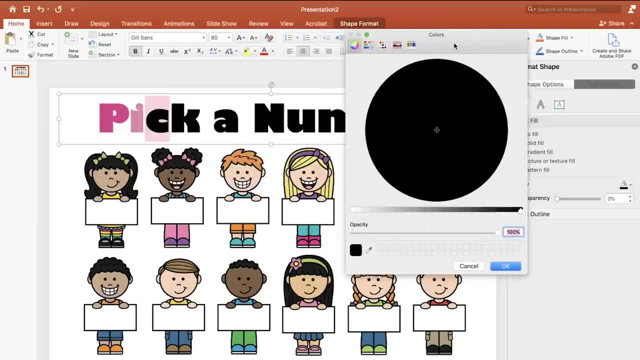 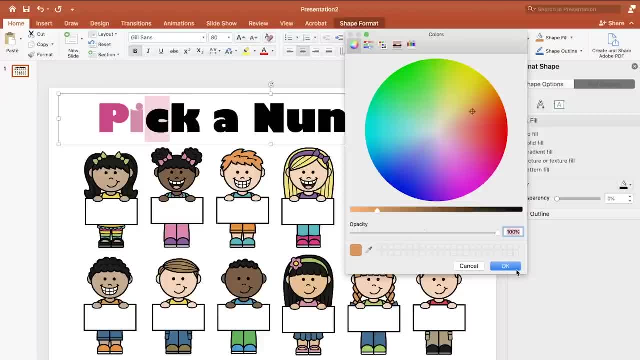 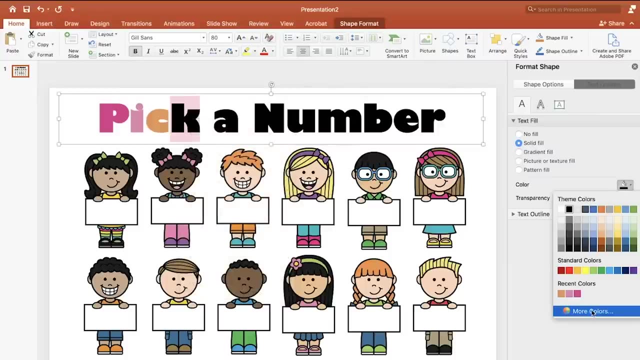 more colors. I'm going to slide this over, choose the little eye droplet and then go to the hair of this boy and after orange I'm gonna choose yellow and I'm gonna choose the yellow from the first girl's shirt, and this way it'll really make the title match the clip art. 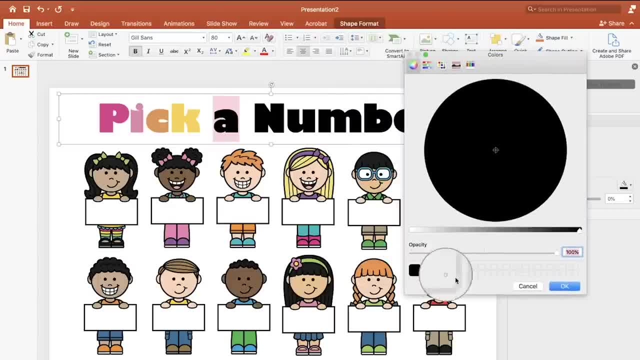 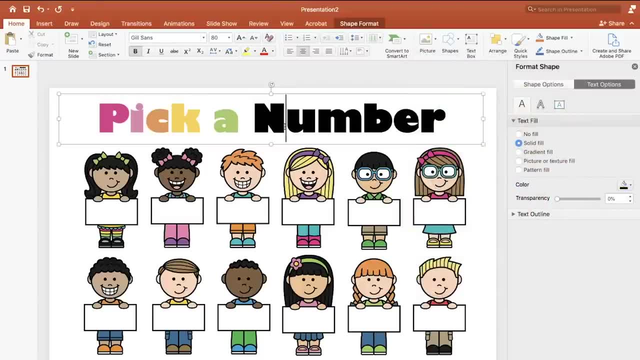 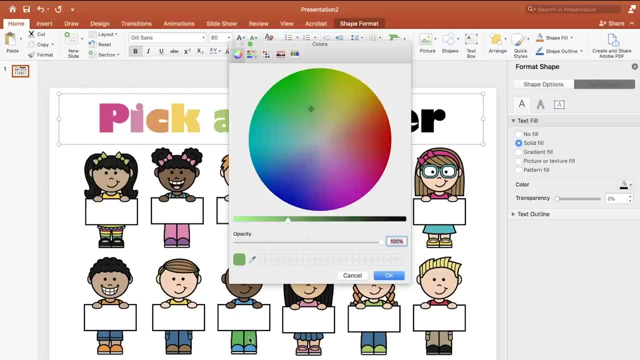 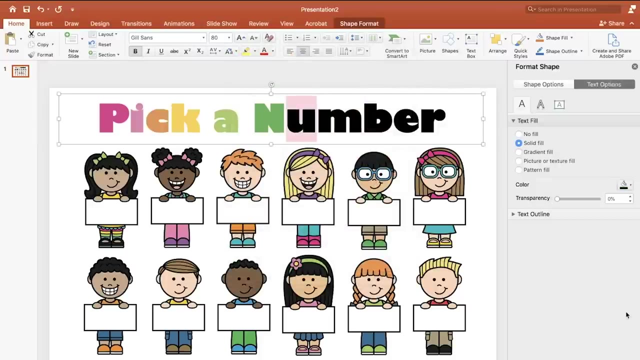 and then then I'm going to go to light green, and for the light green I'll choose the shoes of this little girl. and then I'm going to go to a darker green, For that I'm going to choose the pants of this other boy. and then let's go to blue now, and I'll choose the turquoise from the little girl's skirt. 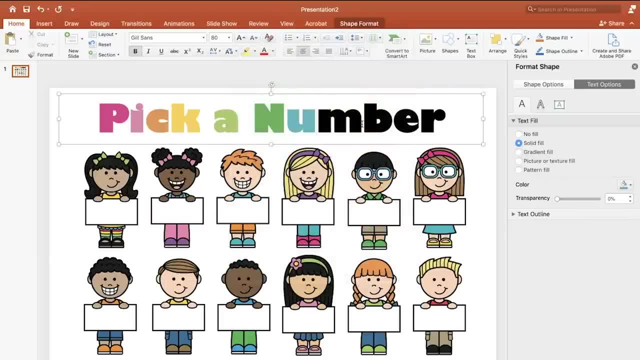 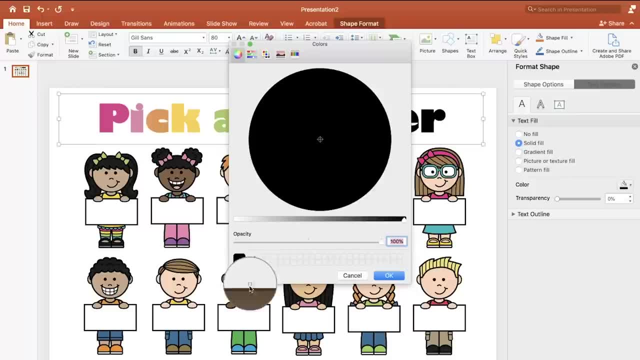 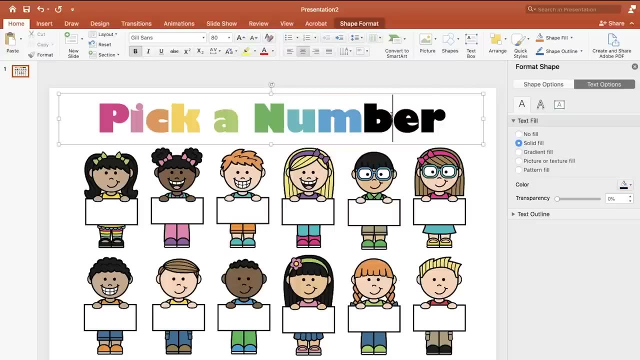 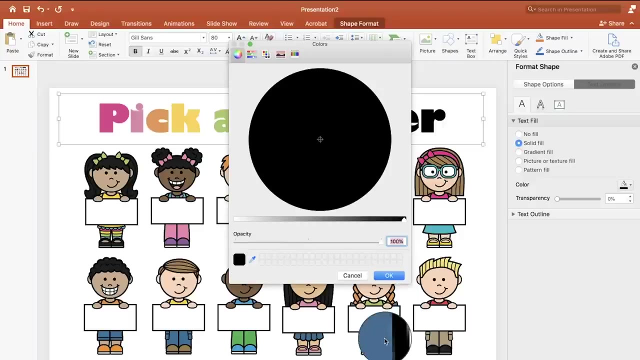 and then I'm going to choose a light blue, and this is very fun to do- I find it very relaxing to do these colors- and then it's starting to look really neat. and then I'm going to go to a darker blue, to that navy blue, and I think I've done all the colors. 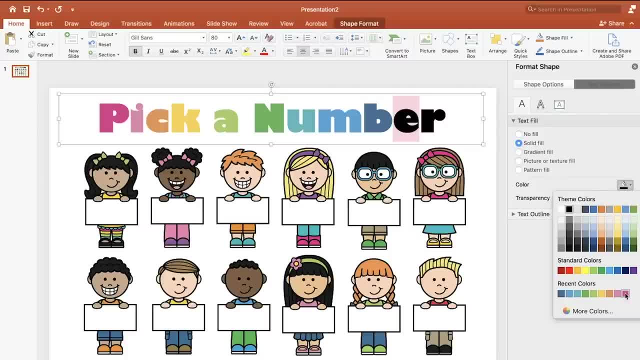 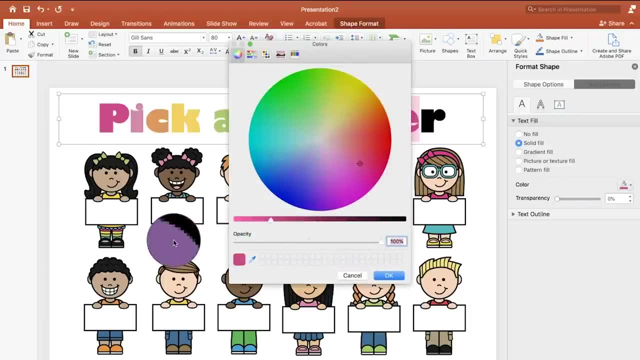 So I'm going to go back to the dark pink, which is one of my recent colors here. that it's saved, Or no. actually let me do purple. I forgot purple And I see purple here on this little girl's shoes. 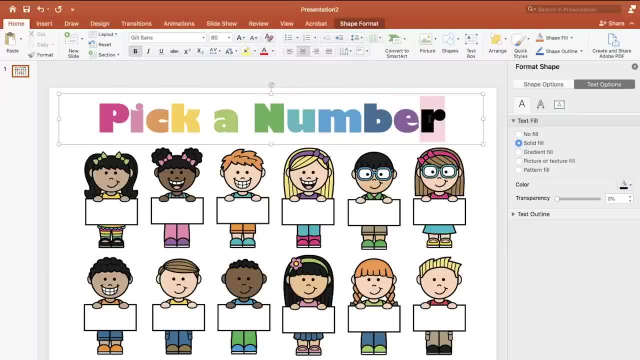 And then now I'll go back to the original pink right there. So that's my title And to make it pop even more, I'm going to choose it. I'm going to make a copy of it. So click Command-C and then Command-V so that you copy-paste it. 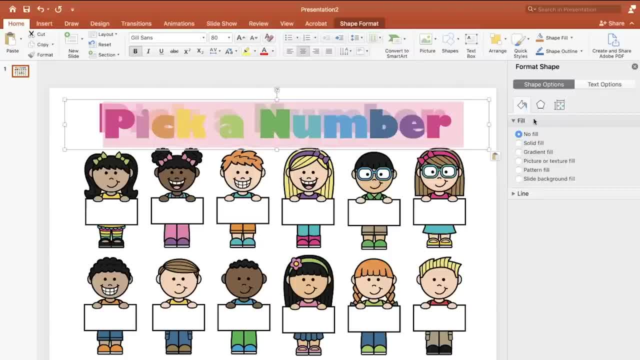 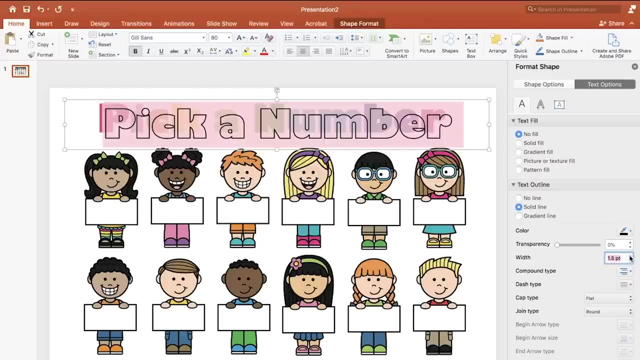 But I'm going to highlight that top one and I'm going to choose- go to text options, choose no fill, but we're going to add an outline, a solid outline that's going to be black And the thickness I'll probably make it 1.5.. 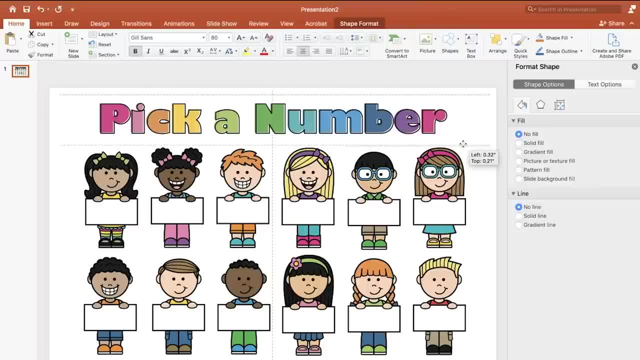 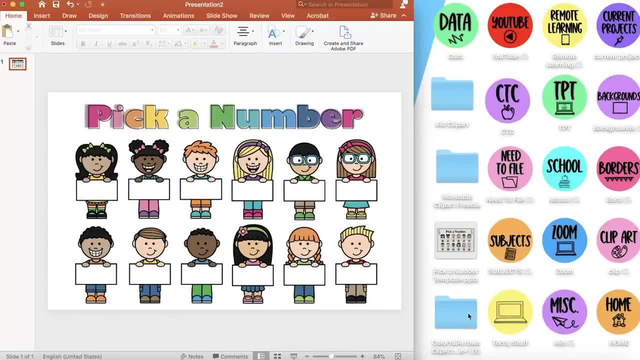 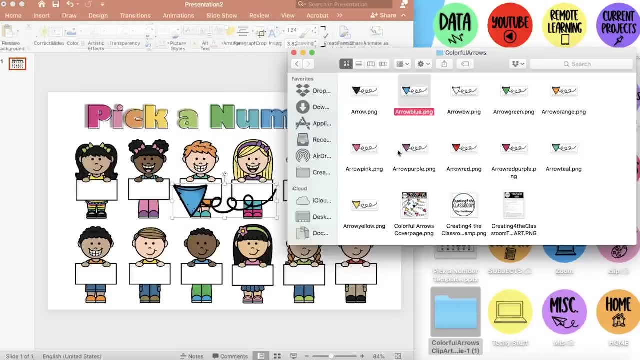 And then I'm going to grab it and put it right there, so you see a little bit of the white and it'll pop up beautiful. I also have some colorful arrows that I want to add, And I'm going to choose this blue and the purple. 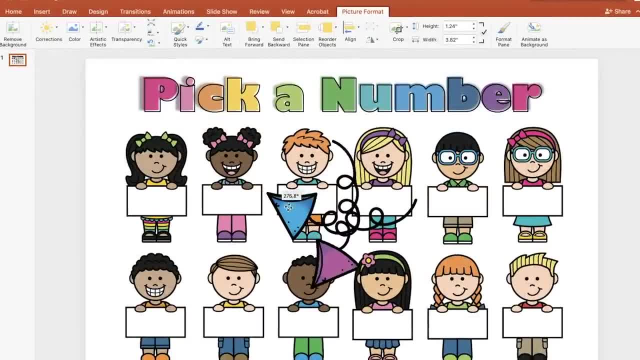 And I'm going to put them on the side just to add a little bit. I'm going to add a little bit of an accent to it. I'll make it smaller and I'll put it on each side. I'll flip this one over. 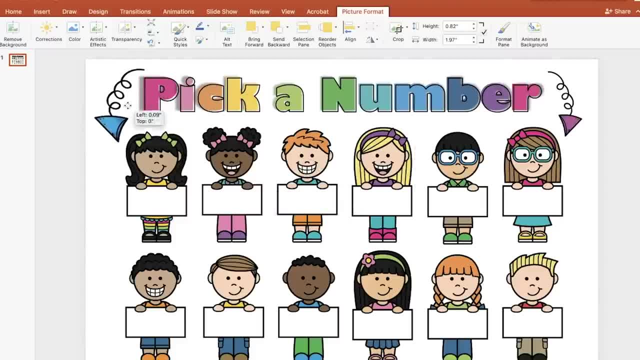 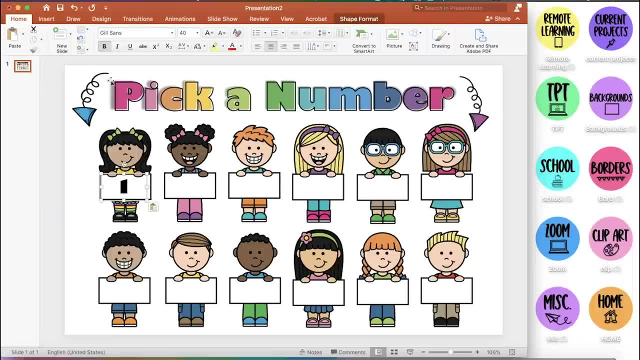 I'll rotate it and add it to the other side. Now we're going to add the numbers to each sign that the kid is holding. And here what I did is I went to Insert and then Shapes, And then you're going to click on the text box, draw the text box and we're going to put the number 2.. 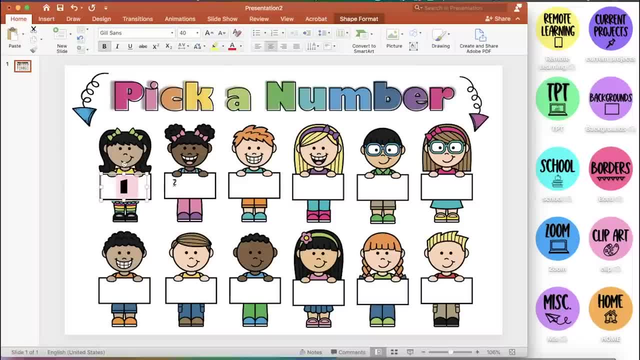 And this is the same font and it's a size 40. So I'm going to center it. click on 40, and choose the same font that we used for the title, Go ahead and center it And to not repeat that process over and over, 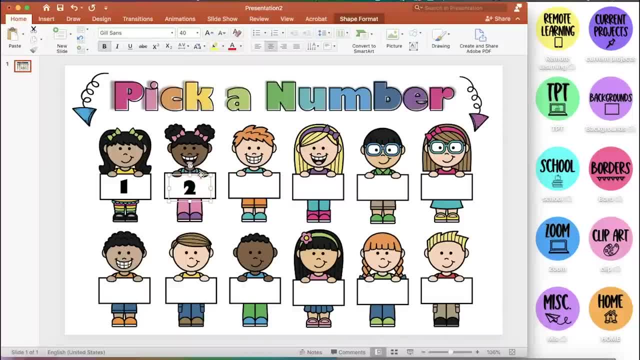 I'm going to click on this box, I'm going to click Command-C and then Command-V for paste, And then I'll just simply change the number And then Command-C, Command-V and change the number, And you do that for all 12 boxes. 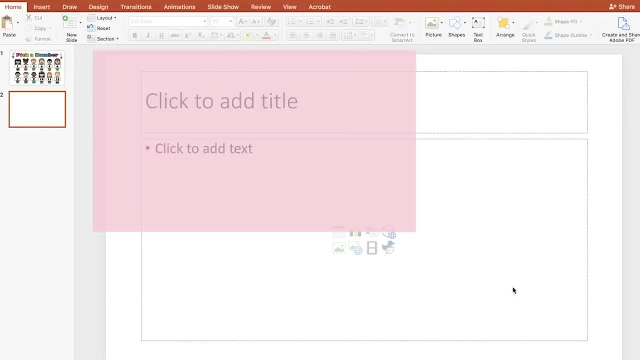 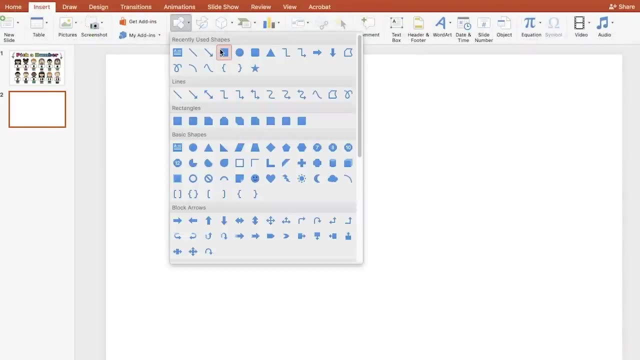 Okay, now I'm going to add another slide. I'm going to erase these boxes and I'm going to add a box by click Insert and then the square, And you're going to draw the square here, not all the way to the end. 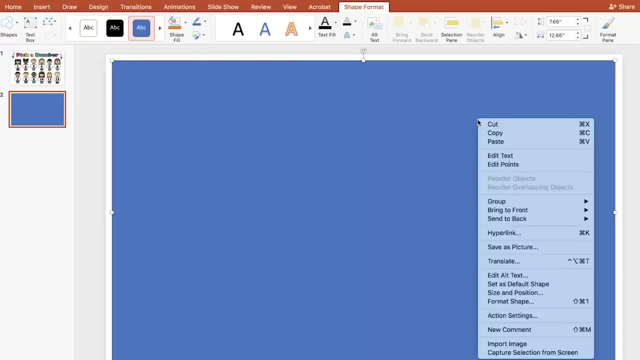 I'll leave a little space on the outside And then where it says text fill, I'm going to add no fill. Oh, it's actually here: shape fill, no fill. And then I'm going to change the color to black and I want it to look thicker. 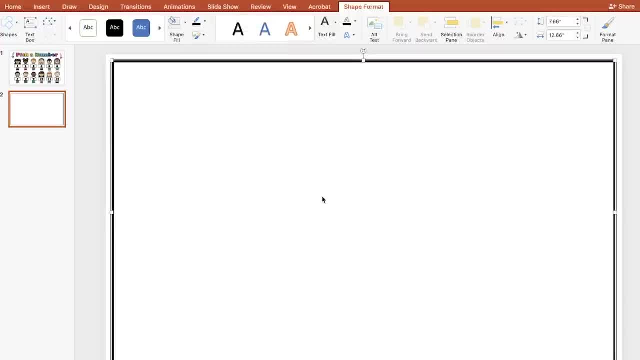 So down here in weight, I'll go down to 6.. I'm going to need 12 of these, so go ahead and go to the left Where you see the slide number 2, click Command and then click on the bottom. 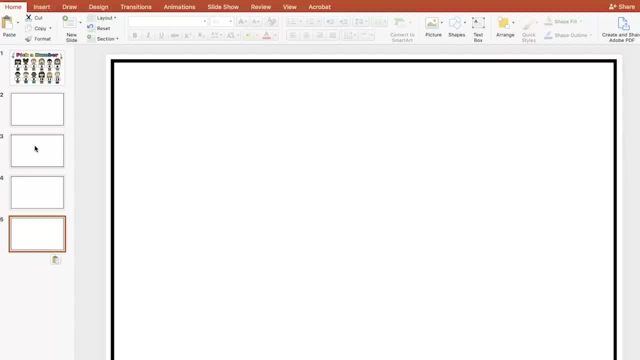 and you're going to click Command-V, Command-V, Command-V all the way until you get to 13.. Those are your 12 boxes, And then we're going to put the numbers for each slide on the corner. Oh, I accidentally copied the little girl. 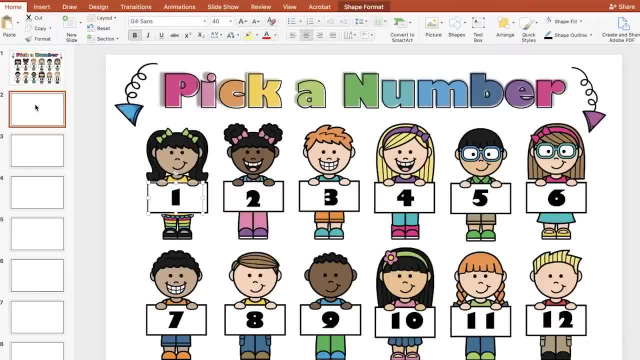 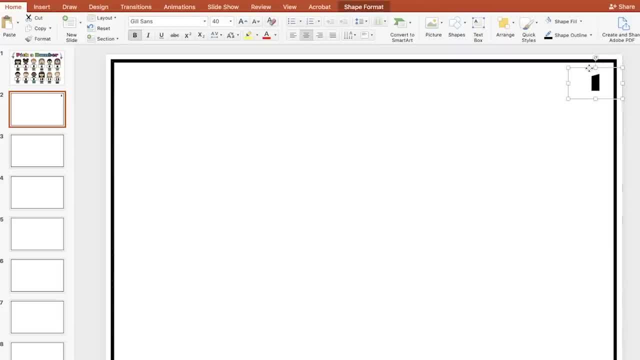 I want to copy the number Command-C And then Command-V. I'm going to put it in the corner And I'm going to also copy this to each slide And then, as you go to each slide, go ahead and erase that and put the correct number. 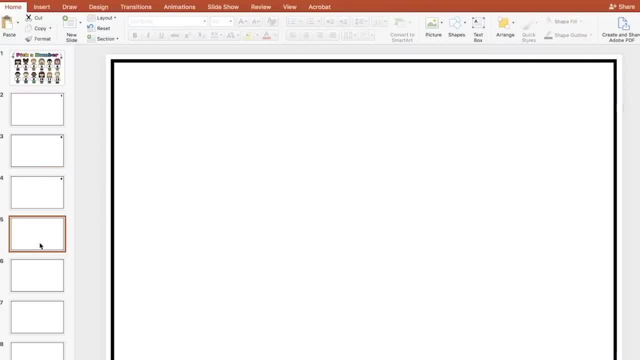 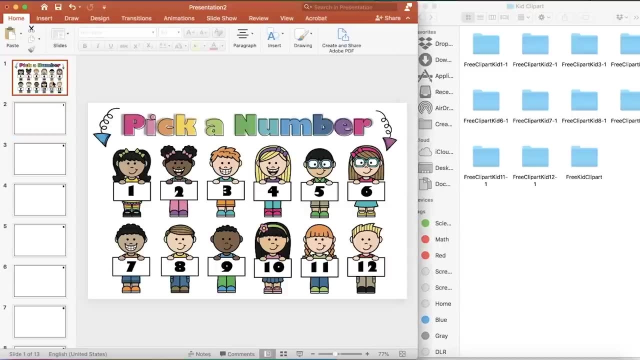 Command-V, Erase it, put the correct number and repeat this step again all the way to 12.. Now we're going to add the same kids in order that is shown here, but we're going to add them for 12.. 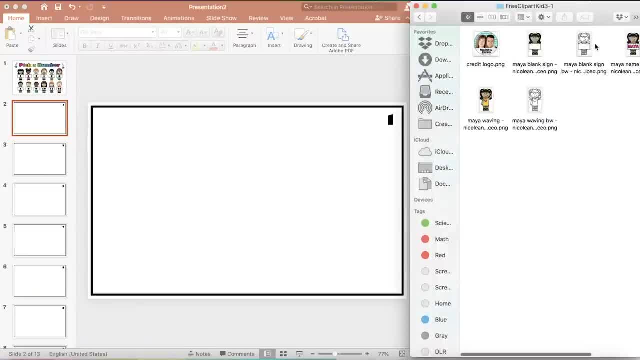 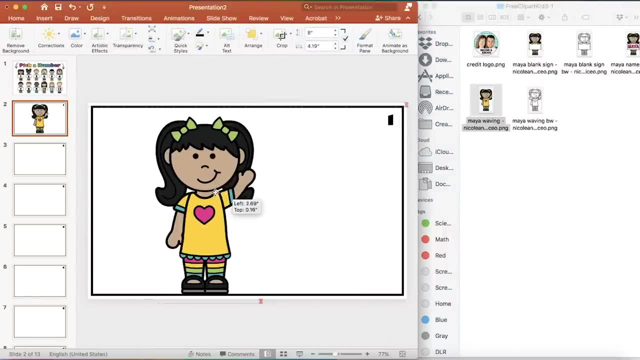 We're going to add them for each slide. so go ahead and open the Clipart and, instead of choosing the kid with the sign, we're going to choose the kid that's waving, And I'm not going to adjust the size, I'm going to simply put it on the side and you're going to repeat this step for every. 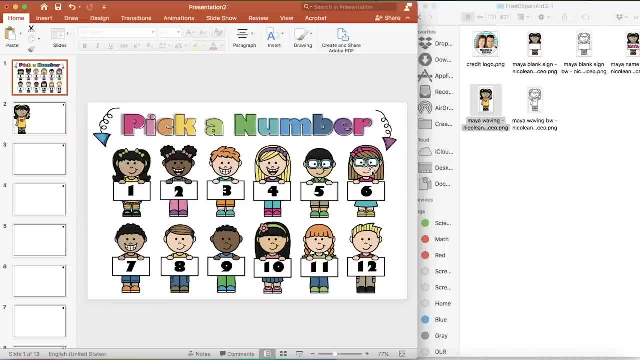 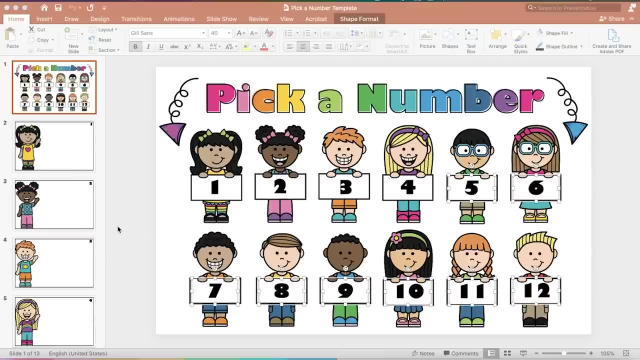 single slide and I'm going to follow the order of the kids the way that it's seen here on this main page. When you're done adding all the kids, we're going to take a screenshot of each page. So you're going to click on Command-Shift-4 to take a screenshot and I'm going to take. 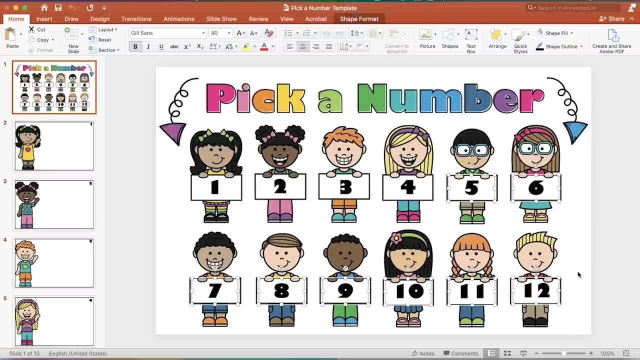 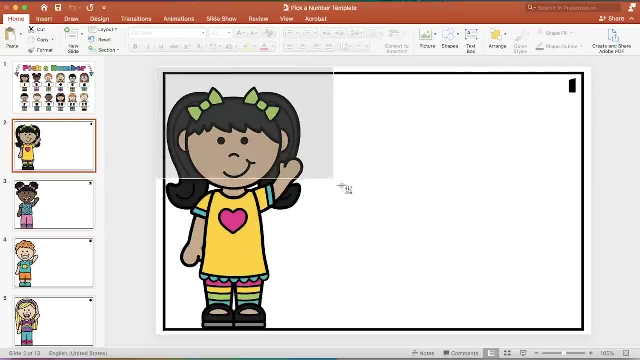 a screenshot from corner to corner. Make sure that nothing is highlighted. You're going to take a screenshot from corner to corner of each slide in order. All of the screenshots are going to go to your desktop if you're using a Mac and you're. 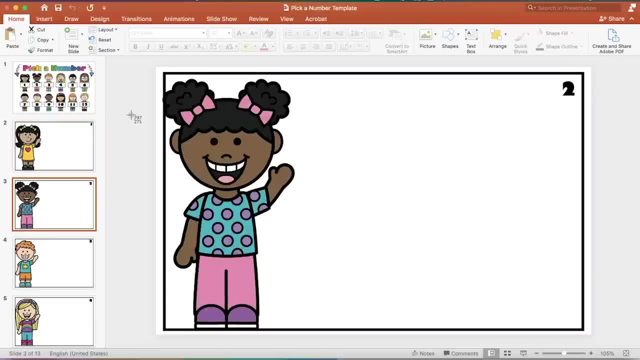 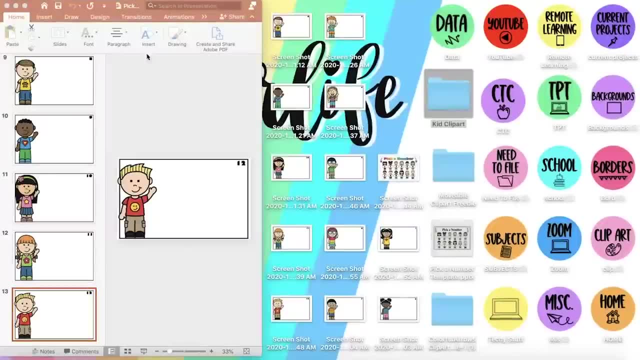 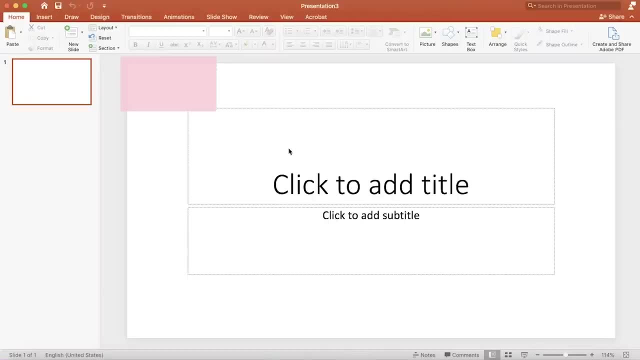 going to follow these steps: Command-Shift-4 for every single slide. You should have 13.. After you have taken all your screenshots- and all of them are on your desktop, you're going to open a new file, a new presentation, and we're going to delete these boxes once. 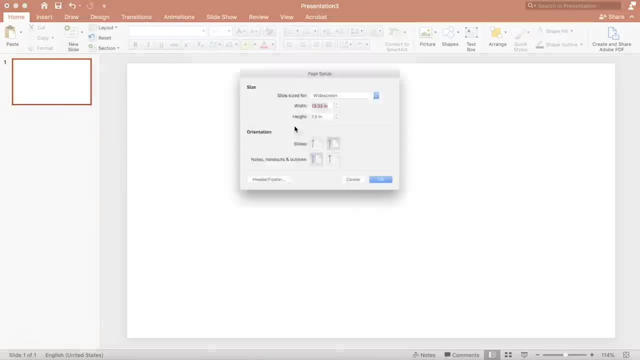 again. We're also going to change the page setup to the previous one, which was 13 by 8.. Click OK and scale down And I'm going to click OK. I'm going to add a few more of these and I'm going to add the screenshots as a background. 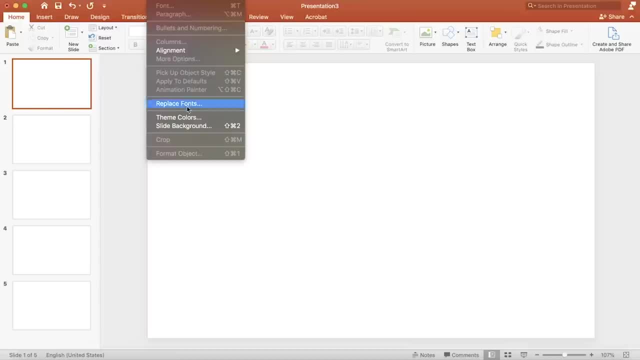 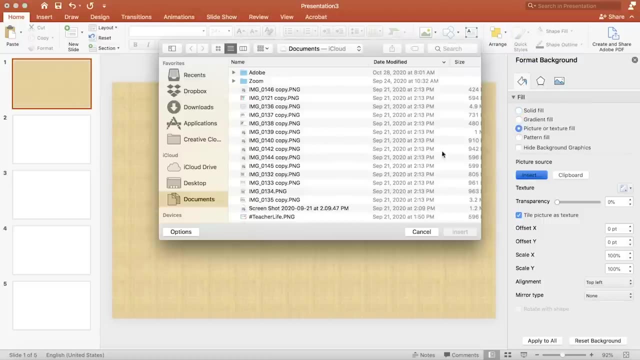 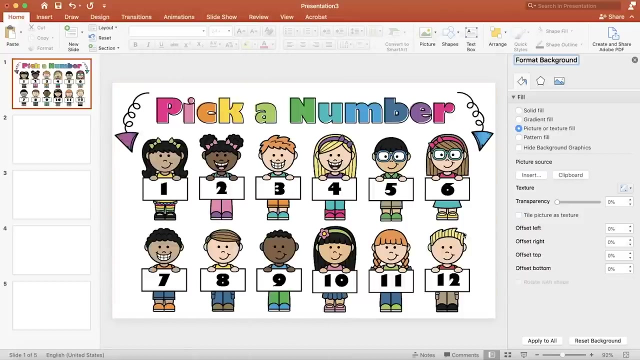 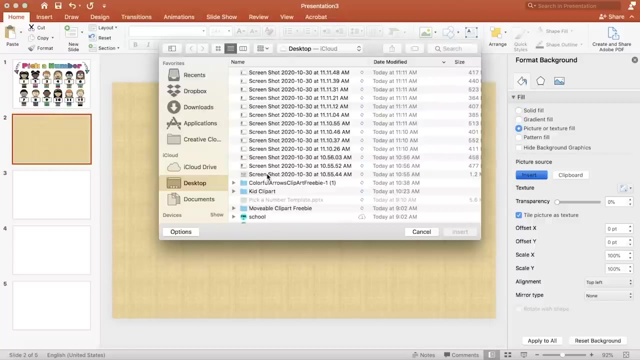 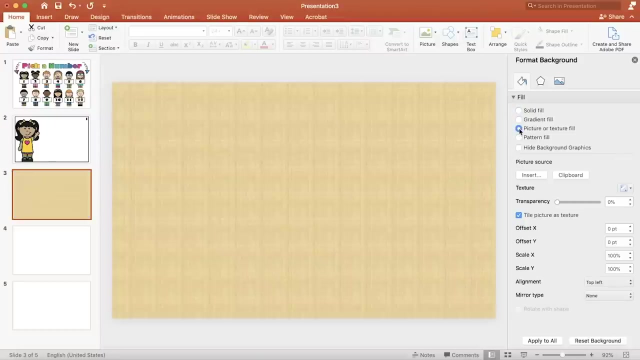 For that you're going to click on Format-Slide Background. Click on Picture and we're going to insert from our desktop the screenshot, and they should be in order. Follow this step. Click on Picture And I'm going to go to the one right next to the previous one and insert. 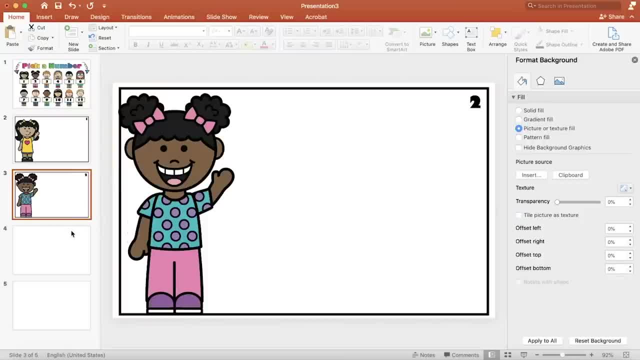 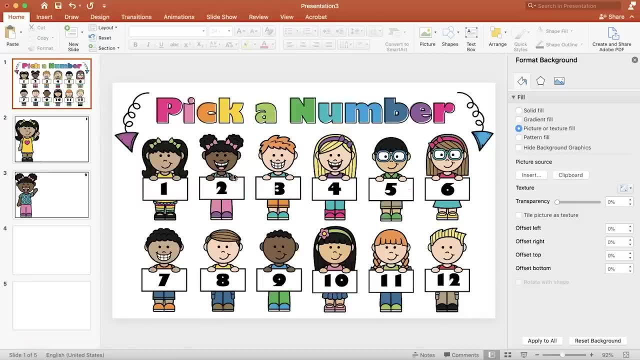 And you're going to follow these steps until you have inserted every single one. When you insert it as a background, the students would not be able to move the screenshot. I mean the clip art that you added, so it would be a background instead. 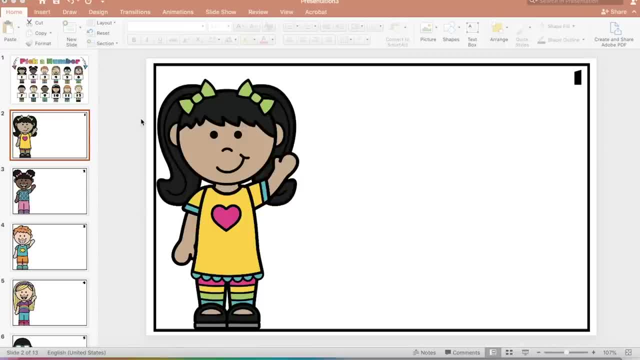 Then you're going to add the profile, Click OK And again you're going to add the questions that you want to quiz your students on or review. You can add a picture, you can add a screenshot from something that you already have like. 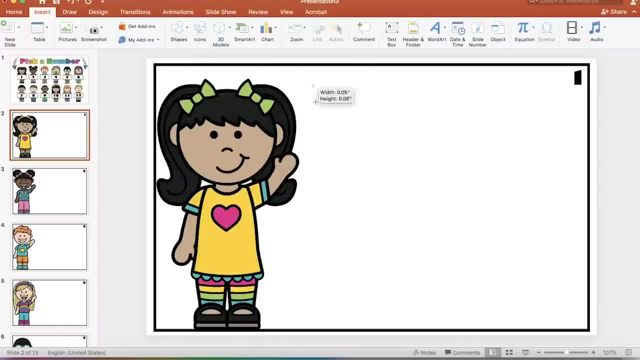 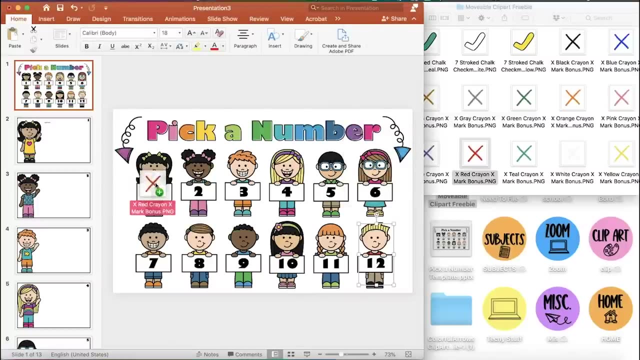 a worksheet, or you can simply just insert text and type your question here. That way, the students have it visible And, like I said, you can design this for however you want to use it. OK, Now we're going to add an X on top of each student. 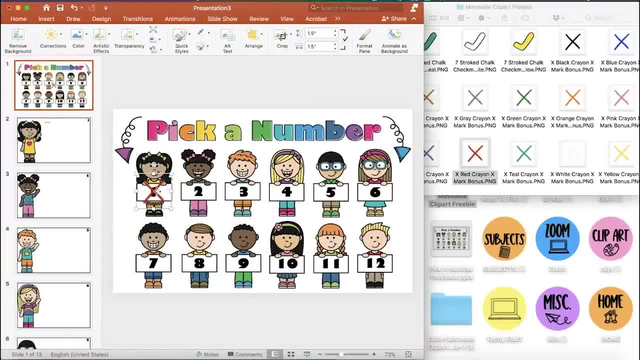 so that it appears whenever they choose that number. And I know you're probably wondering: why are we adding it before? But you'll see how we're going to add animation so that when you click on it this appears. But in order to do that, you have to add the X's before. 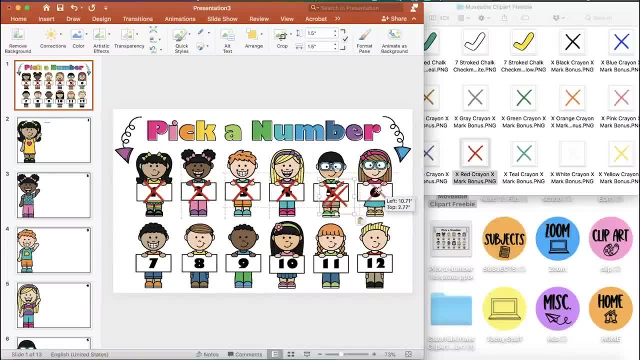 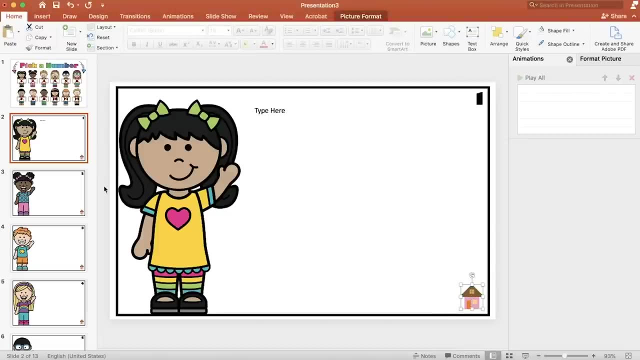 And this clipart that I'm using is movable. That means the creator of this clipart allows for these pieces to be movable, So we're going to follow these steps. for every single number. I also added a home button to each slide. That way, when you click on it, it'll take you back to the very first page, where the students pick a number. 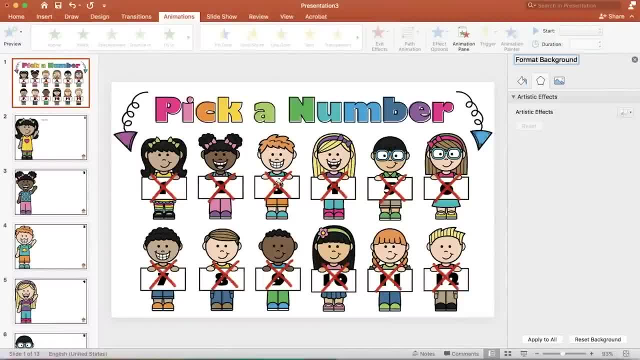 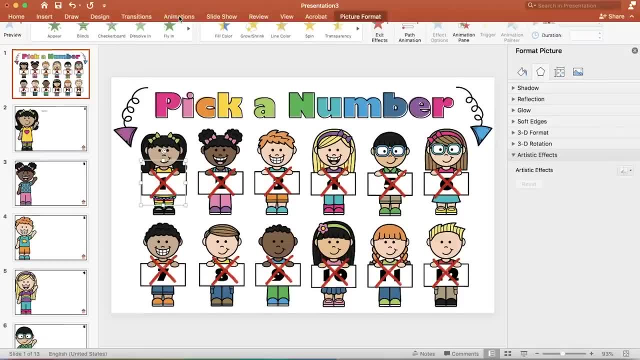 Okay, so I'm going to show you how to link these first three boxes in order. So I'm going to go to this X and I'm going to hit animations And you want to open the animation pane here on the right so you can see what you're adding. 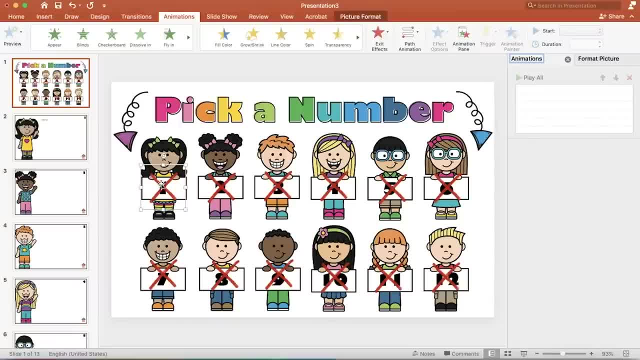 And we're going to program it so that when I click on the clear box that we added, this X pops up. So we're going to click appear And then down here where it says triggers, we're going to click on on click rectangle three. 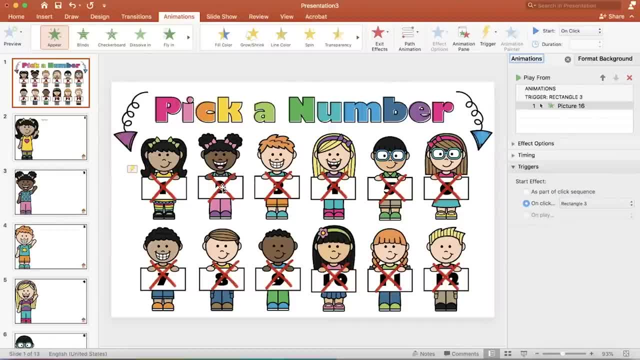 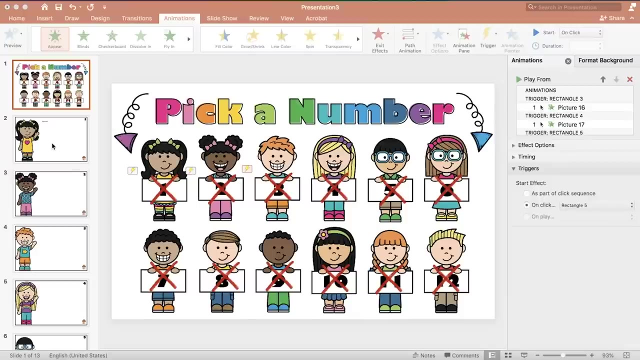 That's the first rectangle that we added, And then we're going to click on this next box and do that, That same step. So click on appear And then on, click rectangle four And do the same step for every single X. Now we're going to go to the home buttons and we want to add an action. 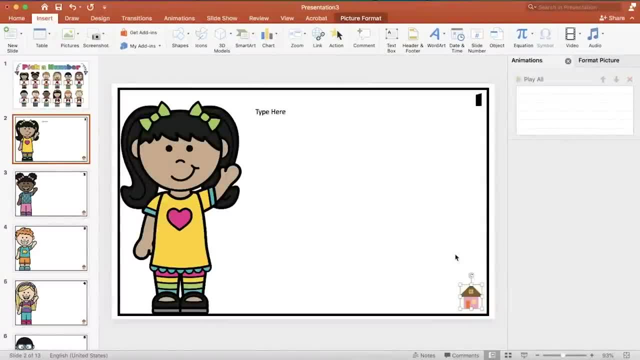 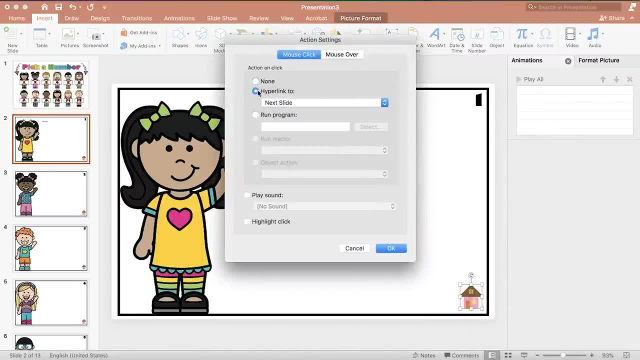 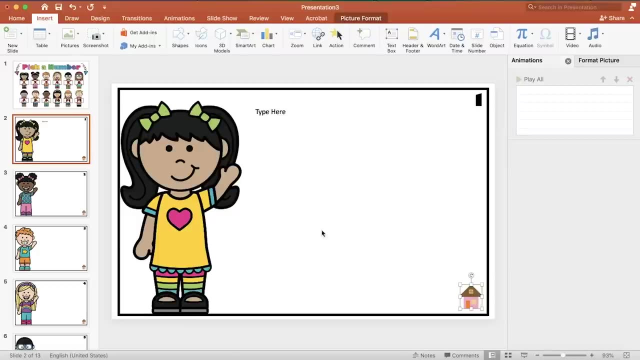 So we're going to go click on it and then click insert, or actually right click it or use your two fingers And click on Action settings, and we want to hyperlink it to go to slide number one. That way, every time you click on that home button, it'll take you to the very first slide. 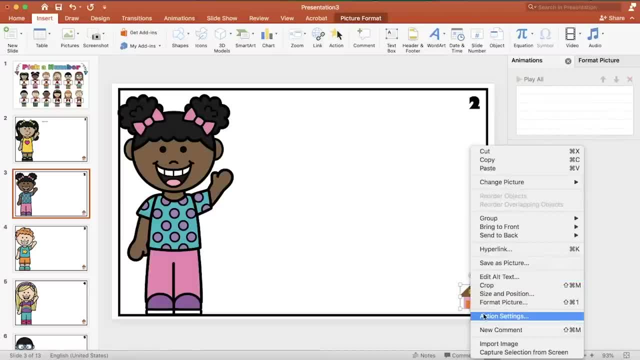 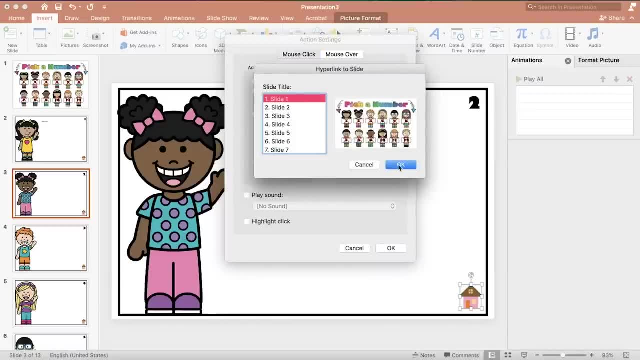 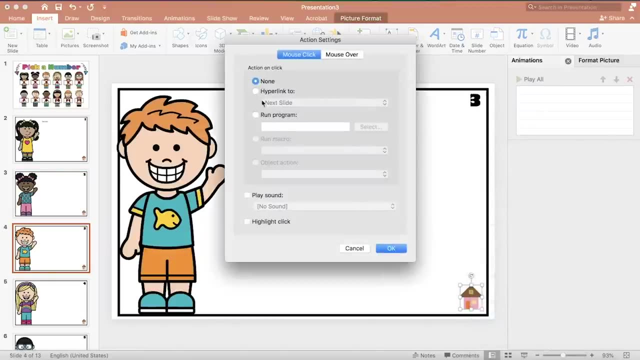 Same steps. Do this for all 12 slides- Action settings, hyperlink slide- and we want to go to slide number one, the very first one. Repeat these same steps: Action settings Slide, Hyperlink Slide And slide one. 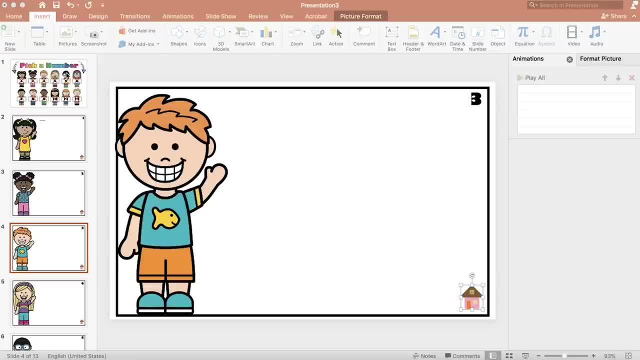 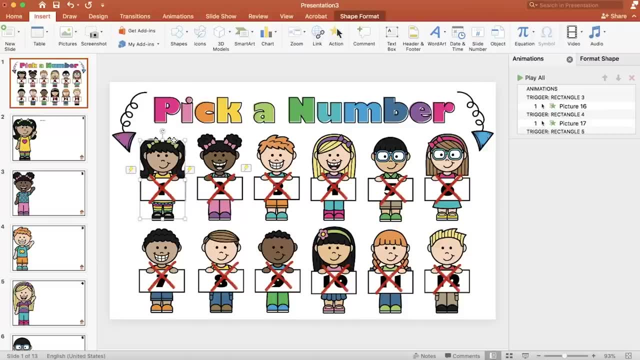 So you'll do that for every single one. Now we're going to go to the very first page and you're going to click on that clear box that you added earlier, and we're going to do the same thing. Go to action settings. 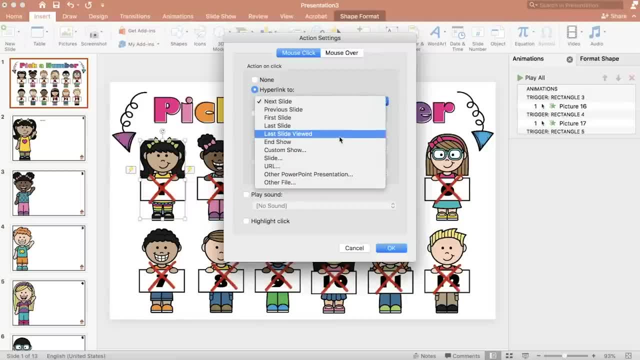 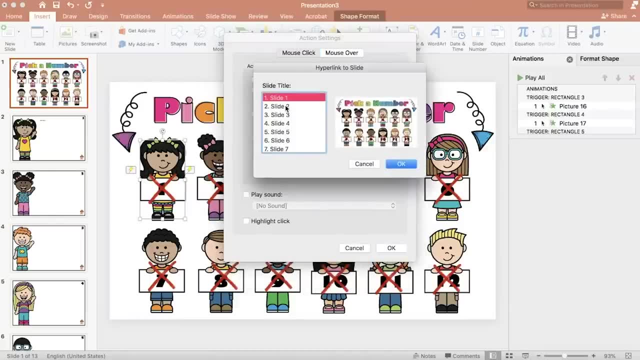 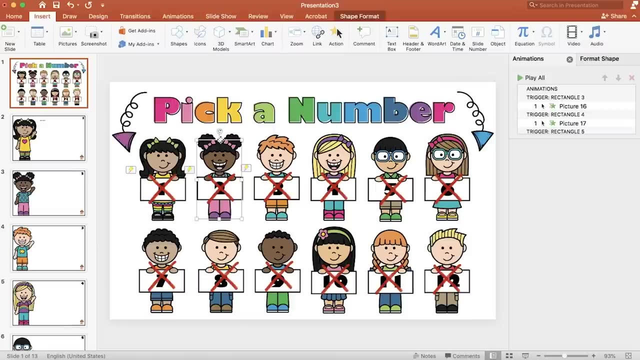 And then hyperlink, And number one is going to be slide two. Slide two going to click on slide and I, every time I click on that clear box, I want it to take me to slide two. so go ahead and hyperlink that and then we're going to go to the next box for the next girl. 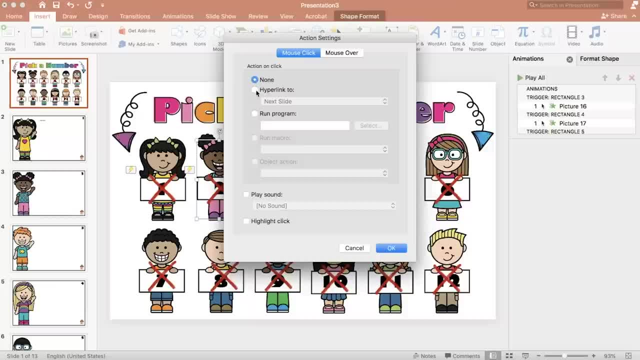 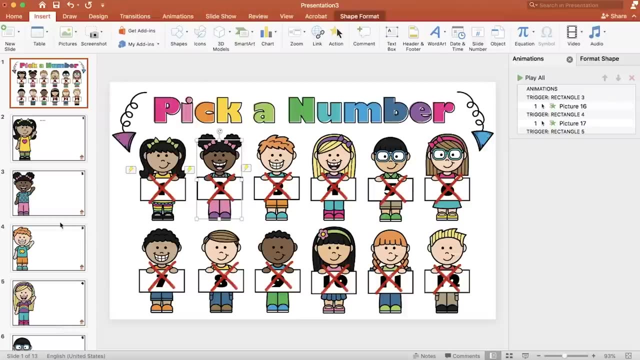 right click action settings, hyperlink, and this little girl is on slide three. click ok and follow those same steps. make sure you're clicking on the correct box. these are all going to have um hyperlinks to different boxes and you'll see here on the left the order of where you hyperlink each one to. 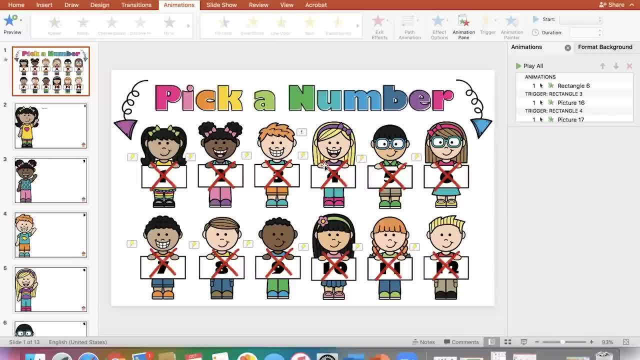 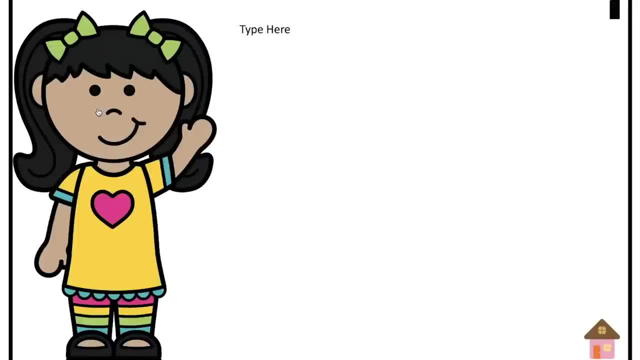 okay. so now that you have coded and you have added all the hyperlinks and animations and you go to presentation mode, you'll see that when you click on a number it'll take you to that slide. you'll have your text here that you have already added, and when you click the home button, 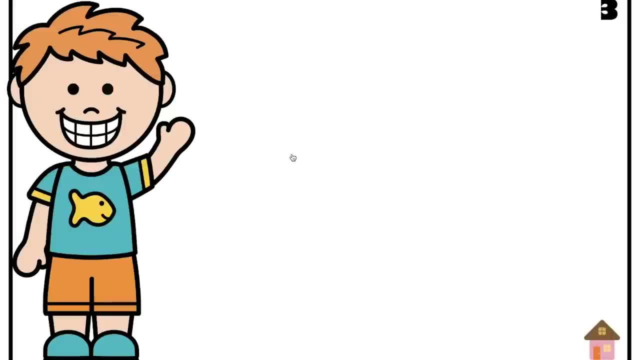 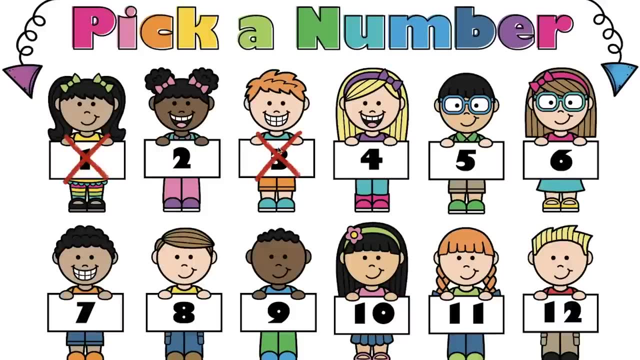 it goes, it adds that x. so no matter what number you click on um, it'll take you to that slide and it'll go back to that main page when you click the home button and add the x. so this is a very neat way for you to review with your students and maybe do a quiz show, or it could be for a morning meeting and each 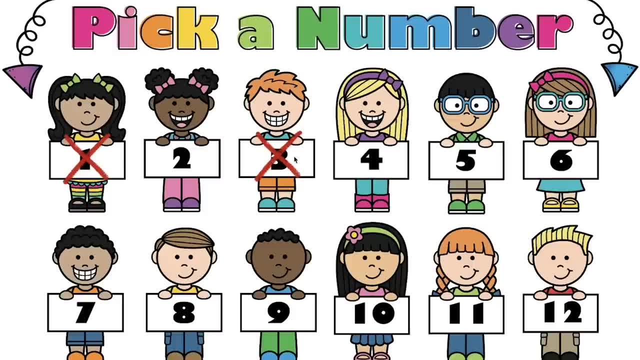 one can have like a question. so be creative and design it the way you want. you can change the clip art and make it your own. so thank you so much for watching. if you enjoyed this video, please hit that like button. if you enjoyed this video, go ahead and like and subscribe and we'll see you next time. with some more teacher tech tutorials.